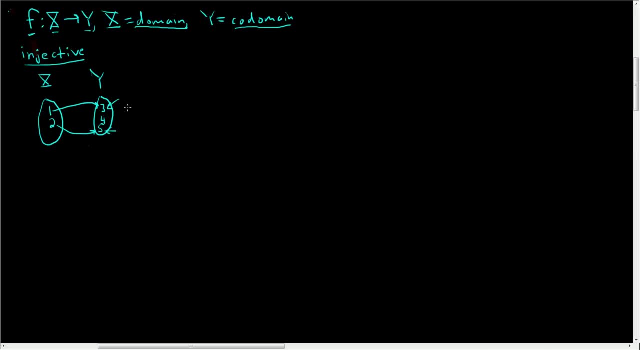 3 gets hit and 5 gets hit. So everything that gets hit gets hit. So everything that gets hit gets hit at most once. So everything that gets hit gets hit at most once. So that's what injective means. 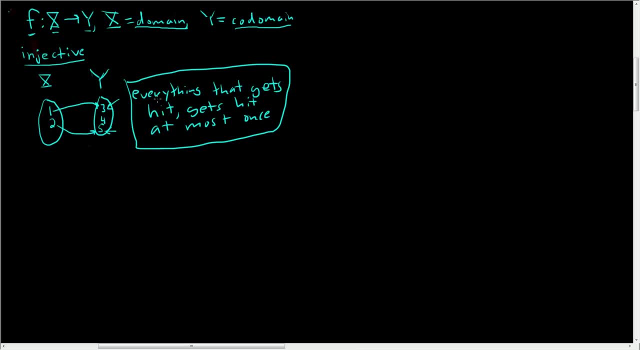 Everything that actually gets hit in the codomain does not get hit more than one time. So what does not injective look like? Let's look at not injective. Not injective would maybe look like this: Here's 1,, here's 2,, here's 3,, 4,, 5, and then 1 goes to 3, and 2 also goes to 3.. 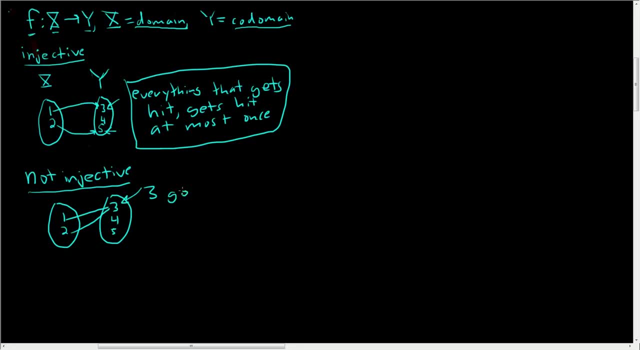 So what got hit twice? 3 got hit twice, So 3 got hit twice. So injective, everything that does get hit gets hit at most once. Alright, now let's look at surjective. Surjective Again. we have. 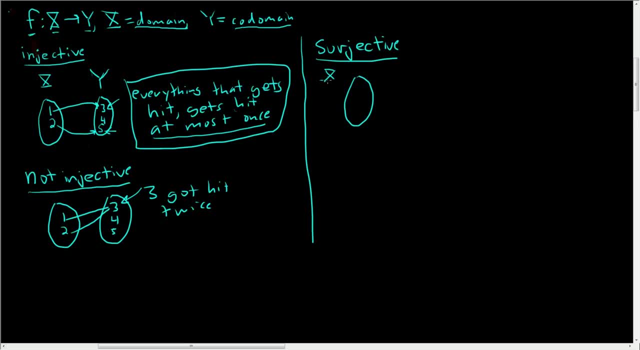 We have capital X, which is here. Let's see, Maybe let's go with 1,, 2,, 3, and over here let's just keep it at 4, 5.. So let's send 1 to 4,, 2 to 4, and 3 to 5.. 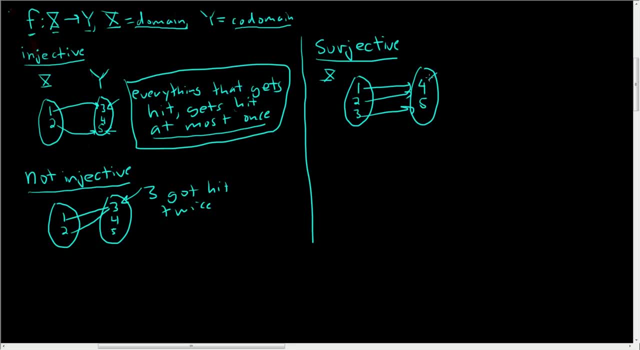 In this case, it's obviously not injective, because 4 got hit twice. right, 4 got hit twice. But you'll notice something: Everything got hit at least once, So everything gets hit At least once. So you want to think of surjective, as everything gets hit at least once. 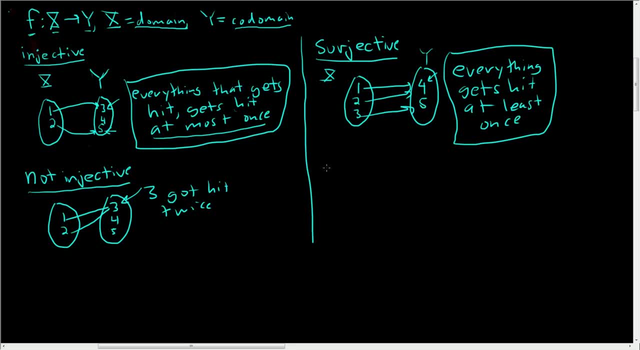 Here's an example of not surjective. Oh, and this was capital Y, So not surjective. So not surjective would look something like this: Here's 1,, 2,, 3, and here's 4, 5.. 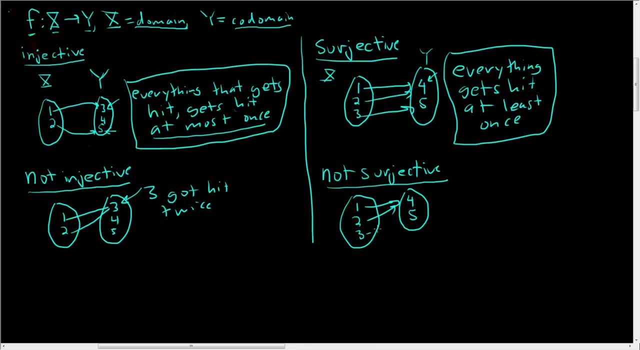 And let's be silly, Let's just send everything to 4.. So what didn't get hit? 5 didn't get hit, So it's not surjective. This is definitely not injective either, because 4 not only got hit once, twice, but thrice.